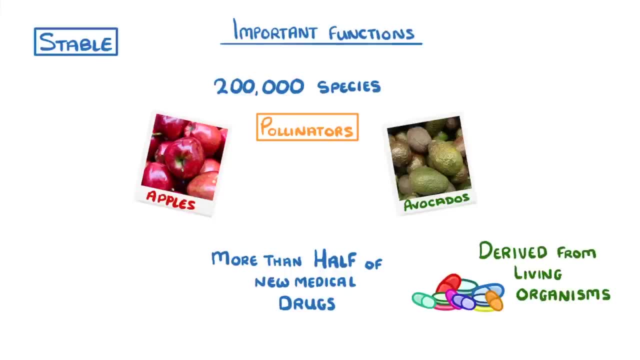 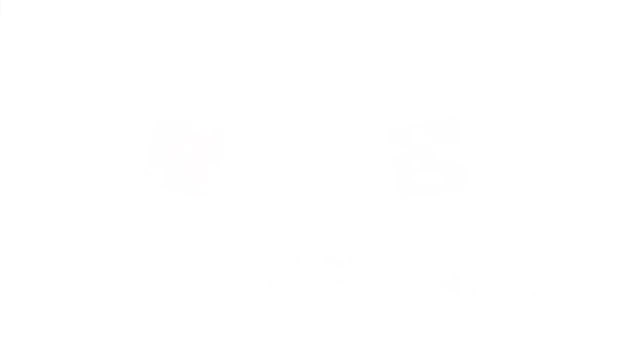 organisms in some way. So if species keep going extinct, who knows what potential medicines we might lose? For the human species to survive and thrive, it's absolutely essential that we have a good level of biodiversity across the planet. Unfortunately, though, we humans have a habit. 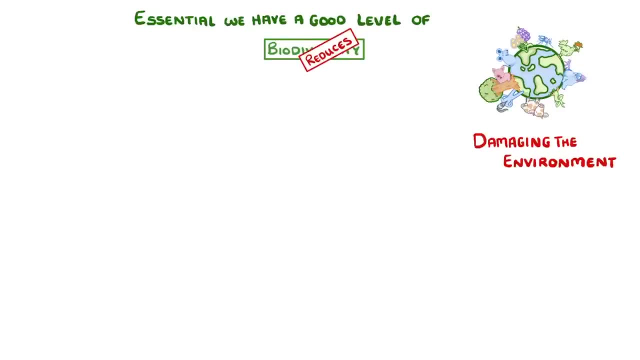 of damaging the environment, which reduces biodiversity, along with all of the benefits that it normally gives us. A big part of the problem is that there are now so many of us. As we can see on this graph, in the past 1,000 years, our population has increased from around 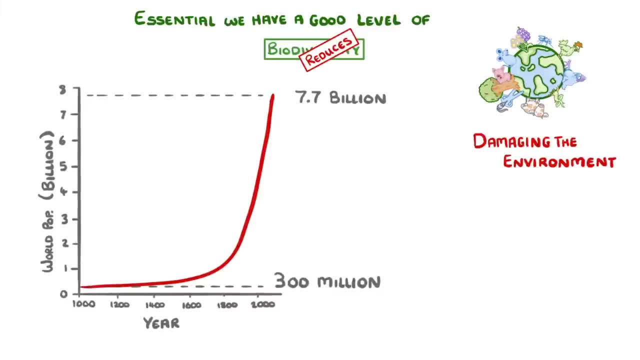 300 million to 7.7 billion. The other part of the problem is that each individual person puts a lot more pressure on the environment than we used to By demanding ever-higher standards of living and consumer goods like new phones, the latest clothes and our own cars. we have to use more, and 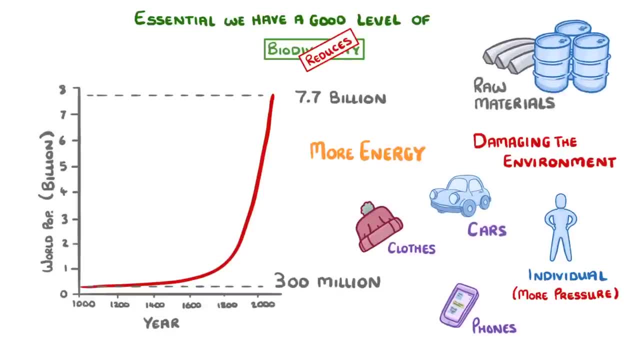 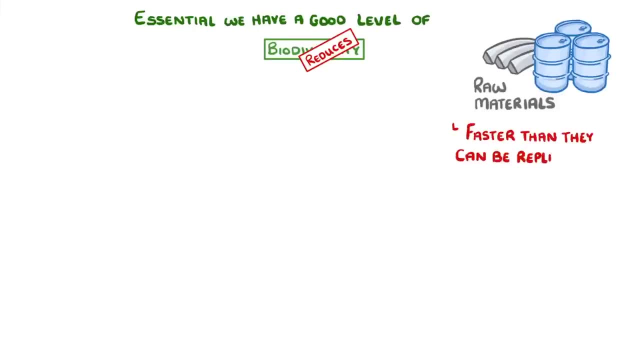 more raw materials and also more energy to put those materials together, Because we generally use natural resources much faster than they can be replaced. we could one day run out of them, just like we drove the western black rhino to extinction by poaching them for their horns. 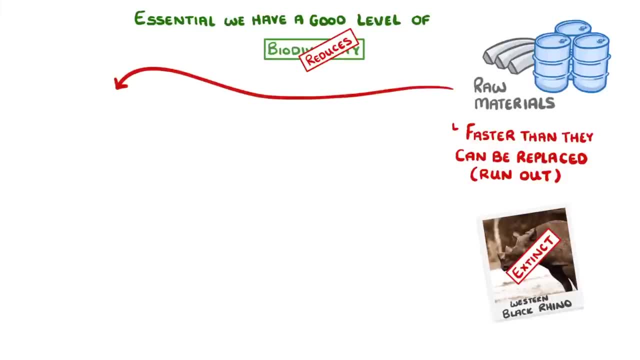 Another issue is that, to get these resources in the first place, we often have to clear out the natural ecosystems that lived there before, which often involves processes like deforestation, which we see in another video. And as if all of this wasn't enough, we also produce loads of waste, both individually. 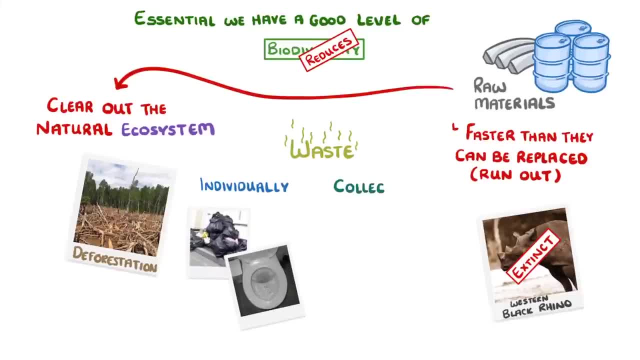 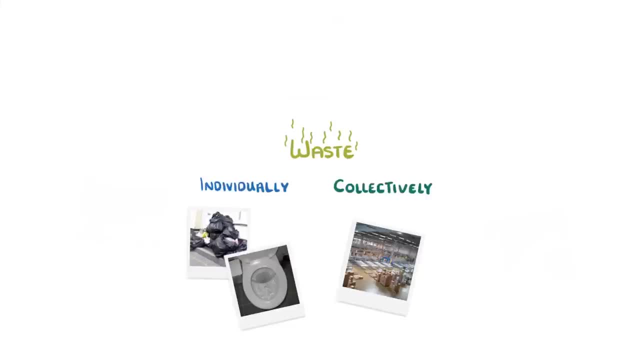 when we throw out our rubbish or flush the garbage out of the water, or when we throw out our waste into the water, or when we flush the loo, and collectively, during the production of all the things that we buy, And one way or another, this waste generally makes its way into the water, onto the land. 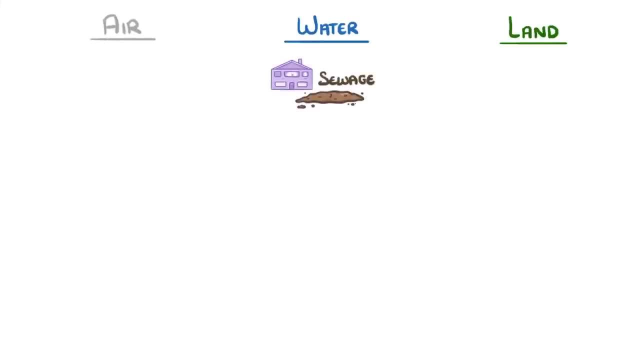 or into the air, For example, sewage from our homes, toxic chemicals from industry and the chemicals used in farming can all pollute lakes, rivers and oceans, which can hurt the plants and animals that live there Meanwhile, even though we bury our household,